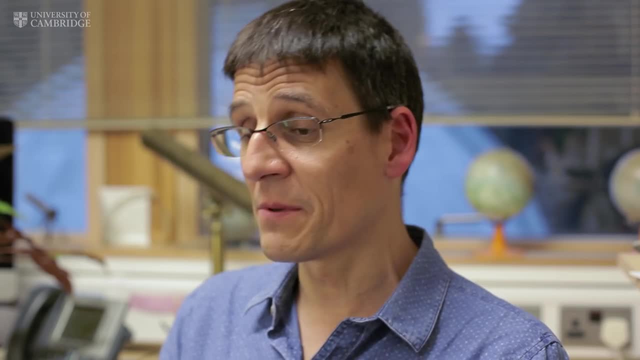 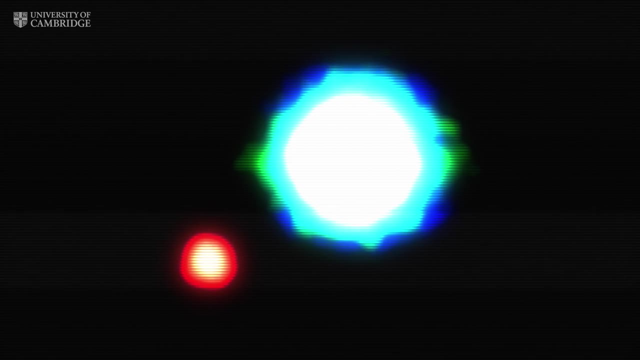 sort it out. And then after some time it continues to be wrong and it becomes so wrong that you have to find out. maybe it's not wrong at all, maybe it's a planet, And then you have to convince yourself. it is the only way to explain this data. 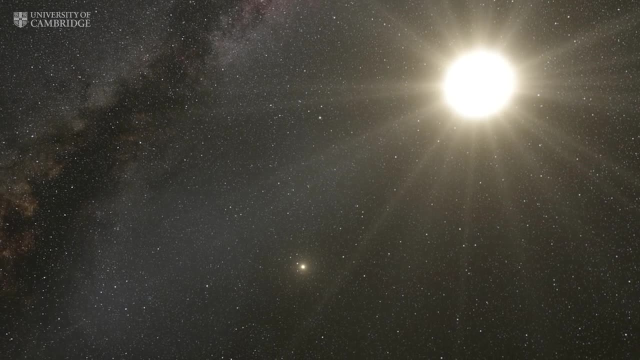 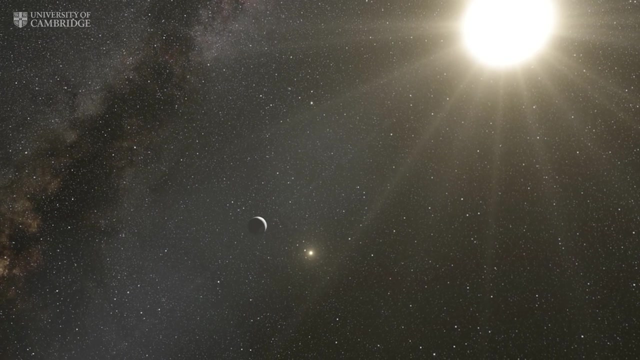 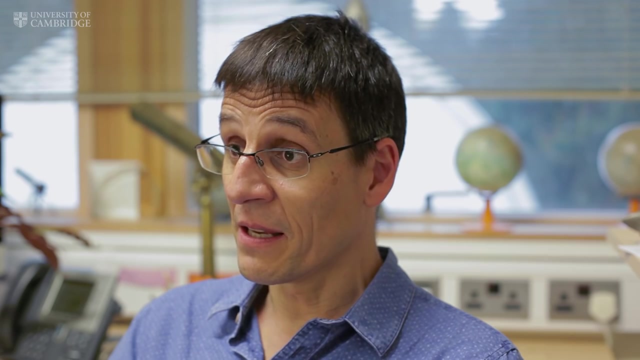 Detecting a planet is quite difficult because the planet is so close to something which is so bright so you get blind when you want to see a planet. So you have to use a trick to find planets, And one of the tricks we are using is when there is a planet orbiting. 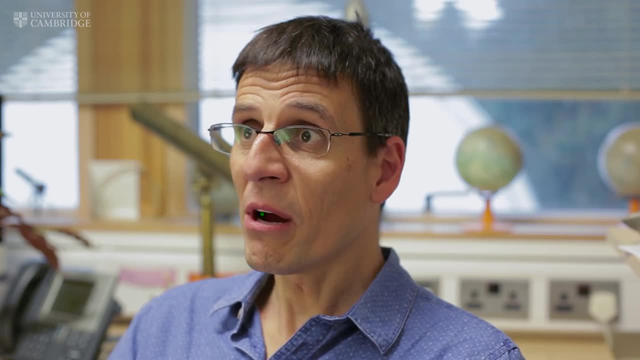 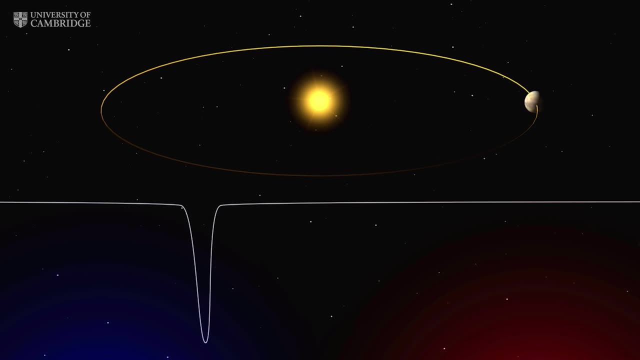 its star. there is something going on on the stars And practically the star is wobbling, changing locations a little bit, And what we could do is we could track the change of the speed of the star. The speed is quite easy to measure because we could use what is called the Doppler effect. 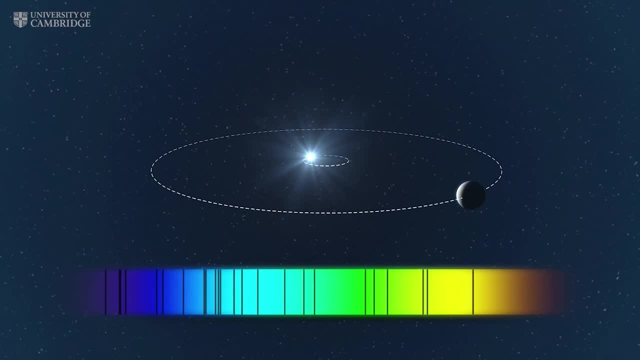 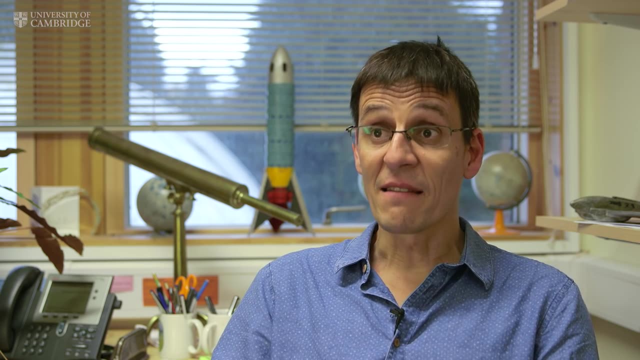 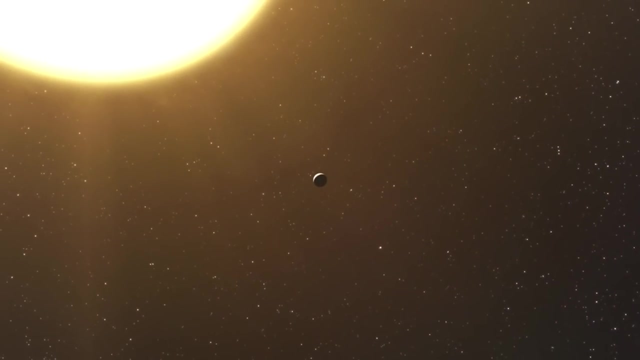 which is the slight change of the wavelength, of the color of the stars. So you use this to detect a change of the speed and then from this you can get if there is something orbiting the stars. In another case we see what's called an eclipse, which is the time the planet goes in front. 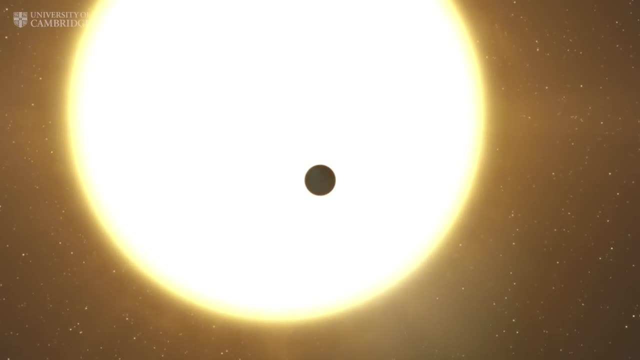 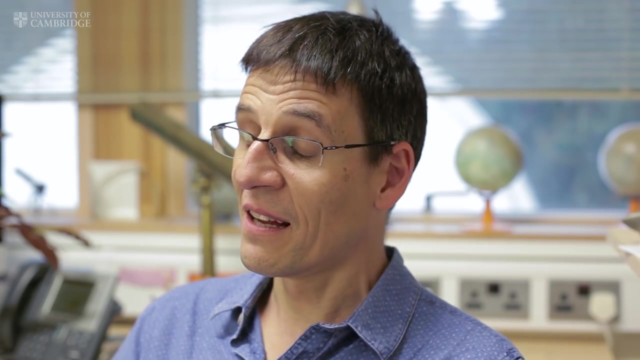 of the stars, making a small shadow in the light of the stars, And from this we can learn a lot about exactly the, the mass of the planet, the size of the planet and, even further, we can even learn something on the atmosphere on some of these planets. 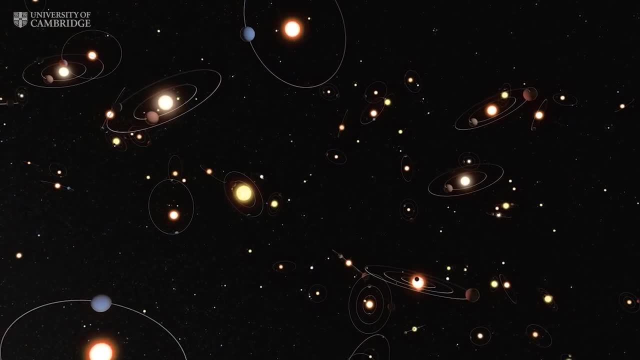 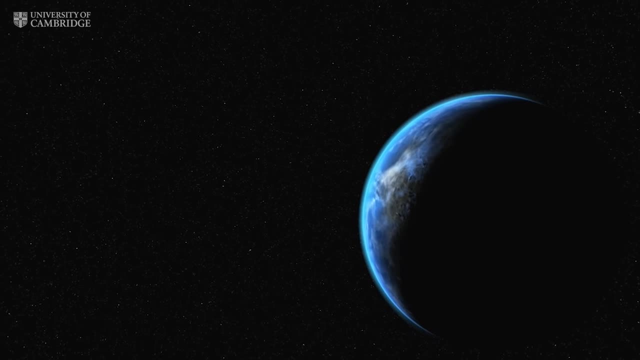 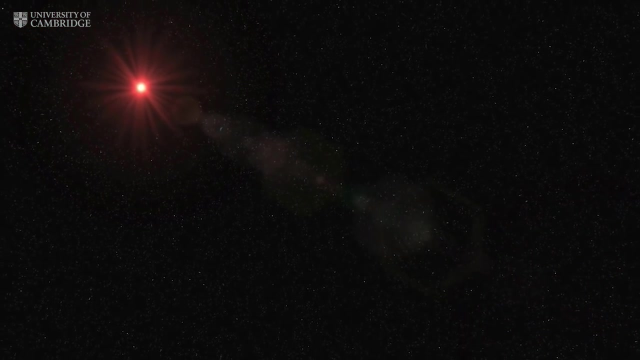 We know that there are about half of the stars with small planets and there is a fraction of these small planets that kind of look like the Earth. but we have not found yet what's called an Earth twin. That is a planet that is exactly the mass, the size and the orbit. of the Earth, And one of the questions we have is: how do we know exactly the size and the orbit of the Earth? And one of the questions we have is: how do we know exactly the size and the orbit of the Earth? And one of the questions we have is: how do we know exactly the size and the orbit of the Earth? 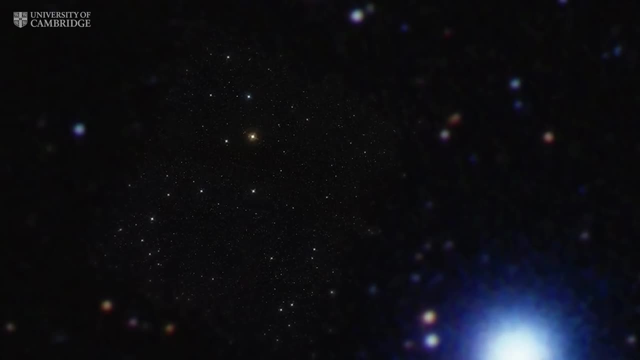 And one of the questions we have is: how are we aware of the size and the orbit of a planet? And one of the questions we have is: how are we aware of the size and the orbit of a planet? The one thing you find a point behind when you find a planet like the Earth is what? 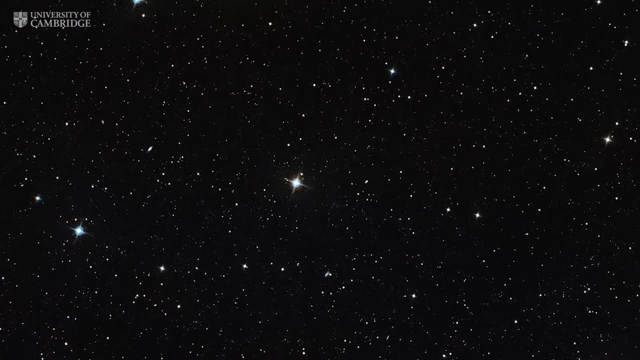 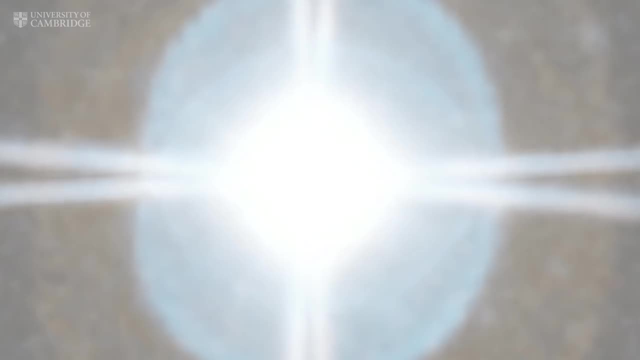 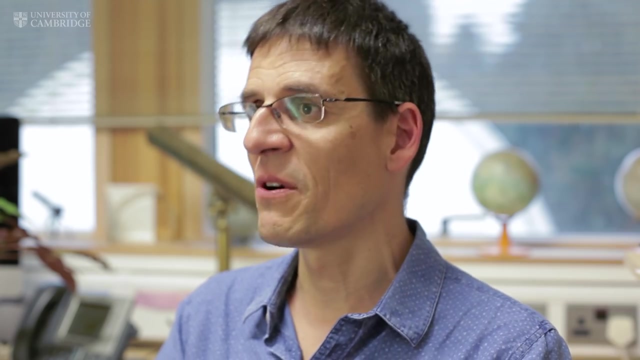 is the prospect of life And what is the prospect that we are alone in the universe? That's a tremendous question, I think, and very profound. Well, my understanding is very unlikely. at least it's not the way that when you've grown up as a physicist, because you tend to believe that anything you have here is. 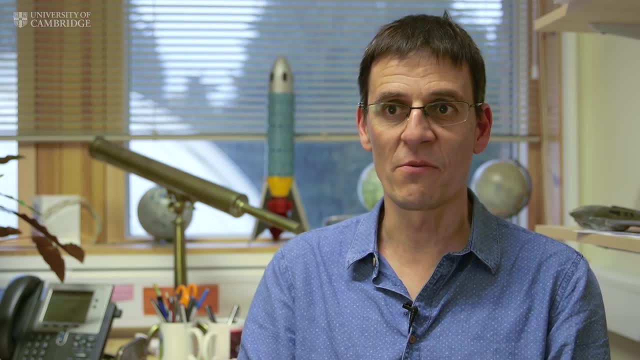 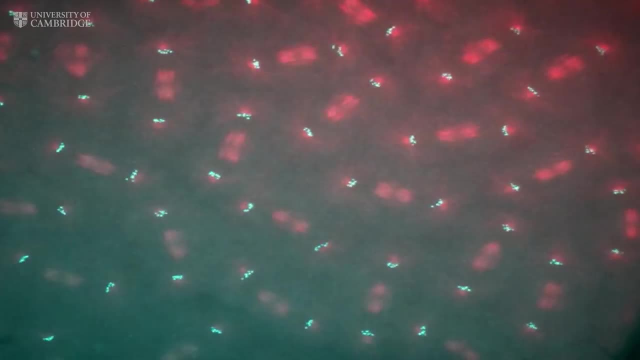 the same elsewhere. So the kind of unique doesn't fit into the rule of physics. but still, if you want to understand life- Well, we know there is life here. It's boring in a way- If you want to understand what is the minimum condition for life, what happens? 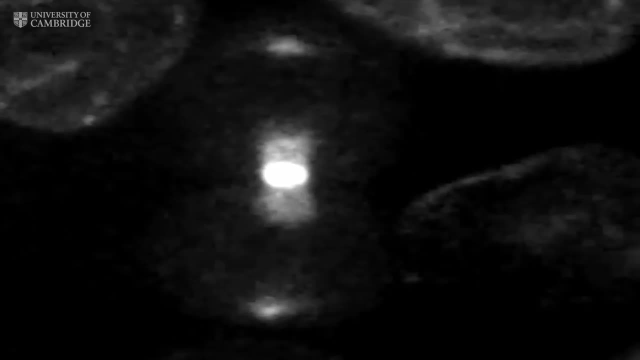 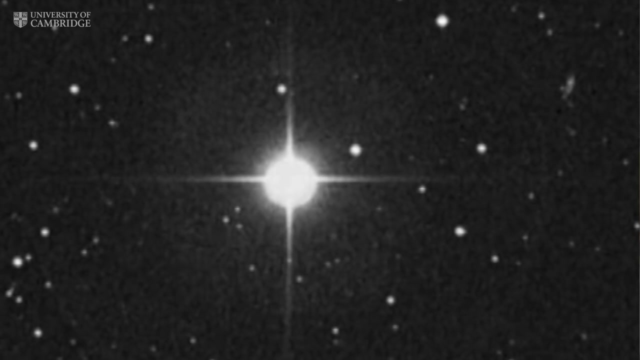 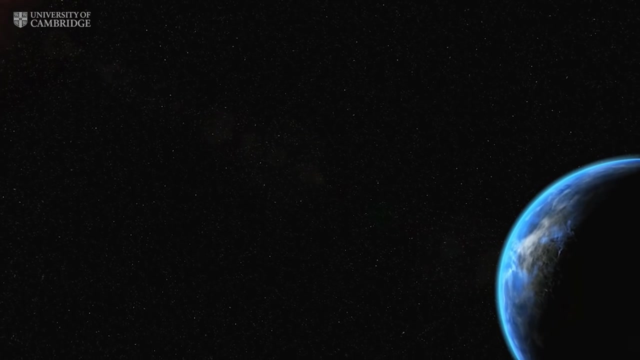 you have to compare with similar other planets. So I think behind this is the life issue, how likely it is to get life. Then the question is: what does it mean life? Well, the kind of consensus these days is water, carbon oxygen. 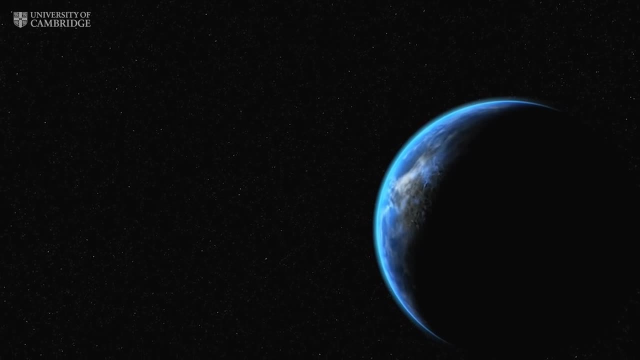 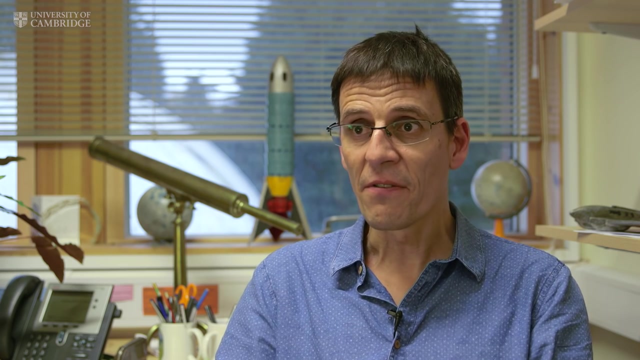 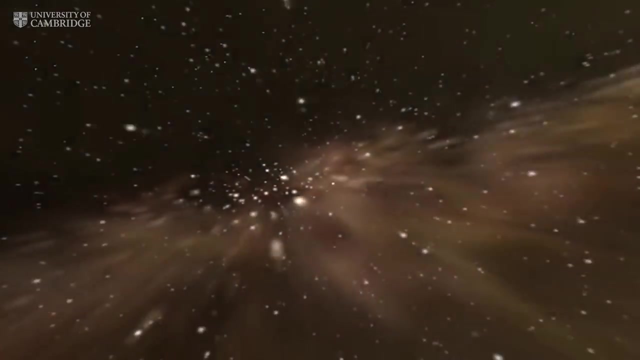 is a very basic element. you find everywhere. There is no something specific here And, according to what we've seen on the Earth is very simple. life seems to be easy to start, But maybe moving from life to something like us is extremely rare. 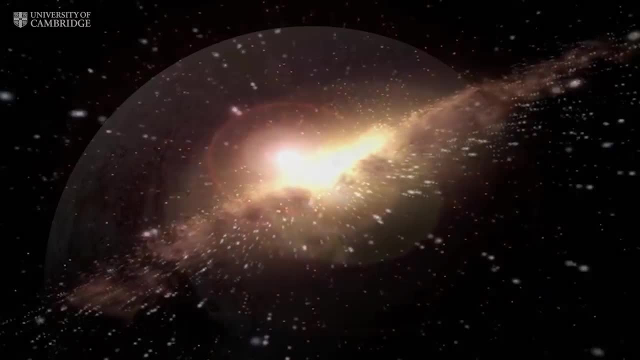 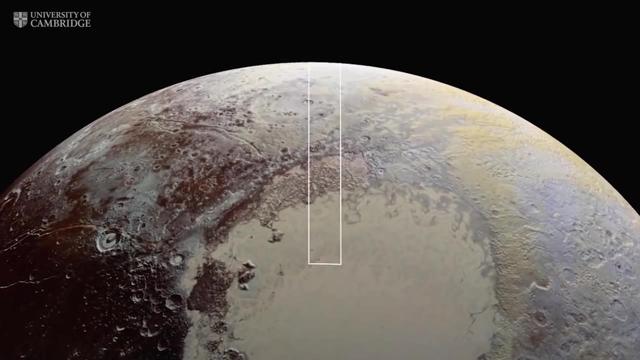 And maybe we aren't the only one on the galaxy. And then, of course, there is always question about: OK, what about life? that would be different. Is it possible to have a life that we just don't detect and we don't see on Earth? 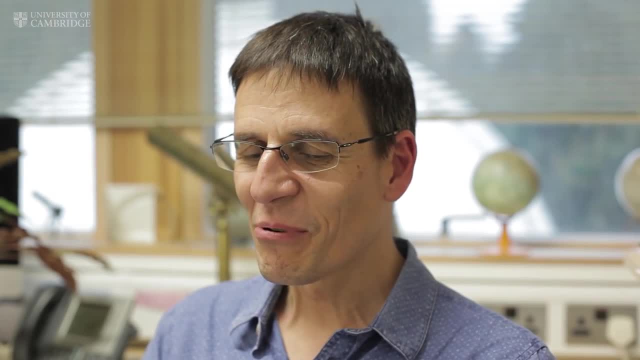 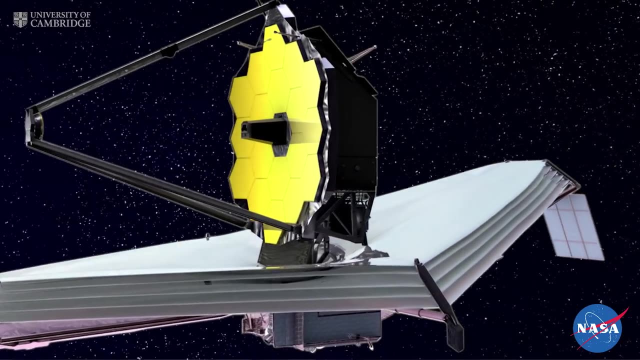 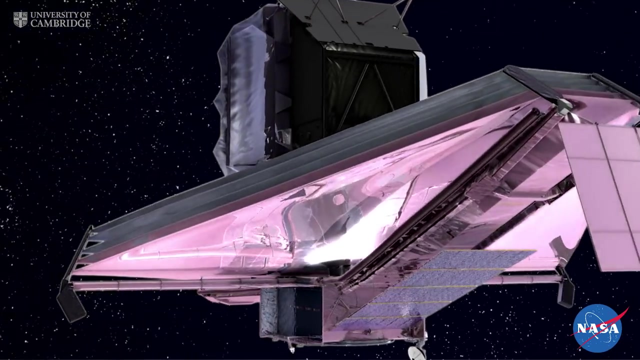 Well, predicting the future in science is a very difficult exercise. We know the equipment that will be available soon, And we have a fantastic machine which is called the James Webb Space Telescope. That will be a kind of a Hubble Space Telescope, but with bigger mirror, with bigger capability. 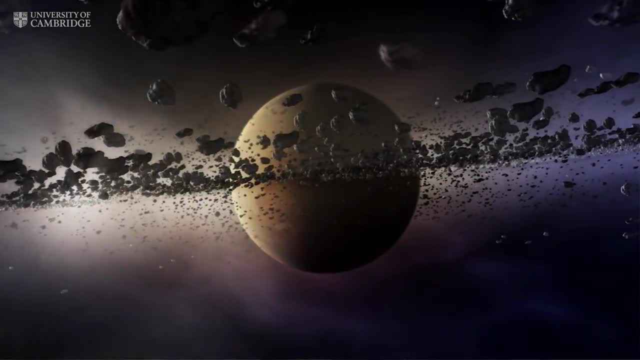 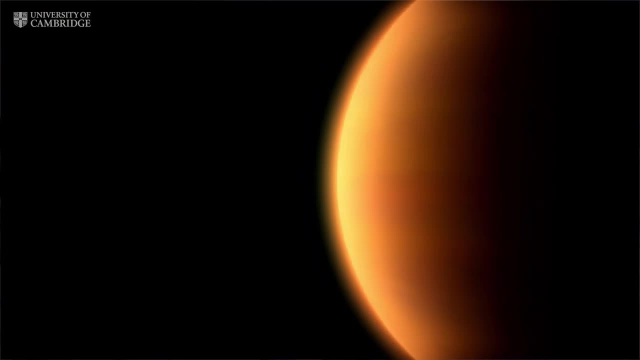 And with this, if we have the right target, we may be able to analyze some of the atmosphere of these small planets, With the secret hope to detect interesting molecules. So what are interesting molecules for us? Well, one of them is water. 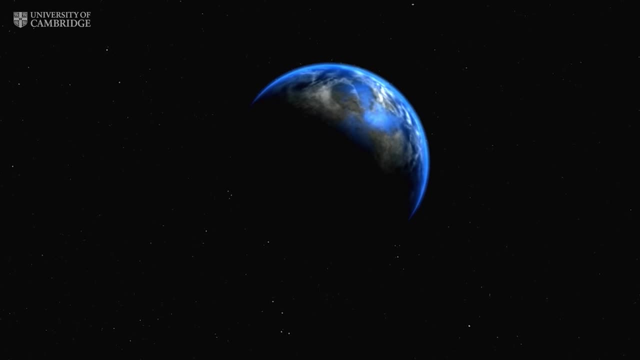 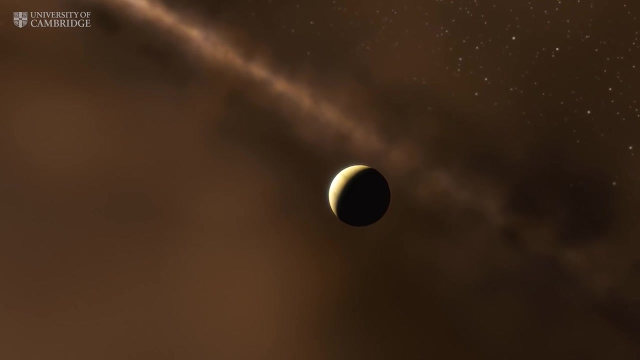 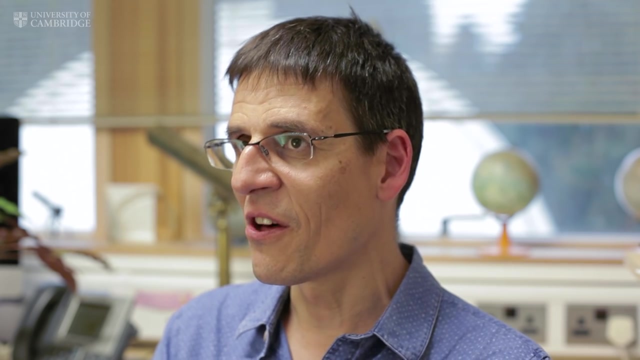 The other one could be a complex carbon-oxygen molecule, And then ozone could be also very exciting there, And anything that can tell you that there is something going on in the atmosphere in a way that is out of equilibrium. Life is something that affects the kind of steady state of the atmosphere of a planet. 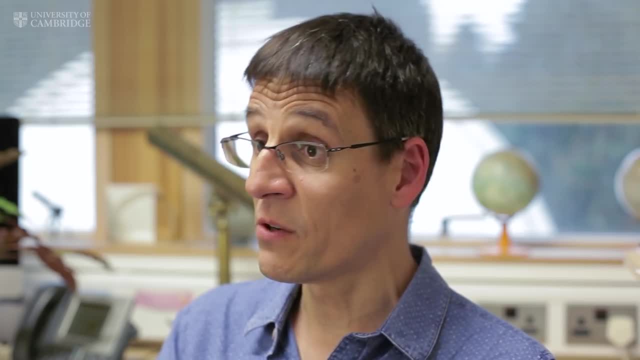 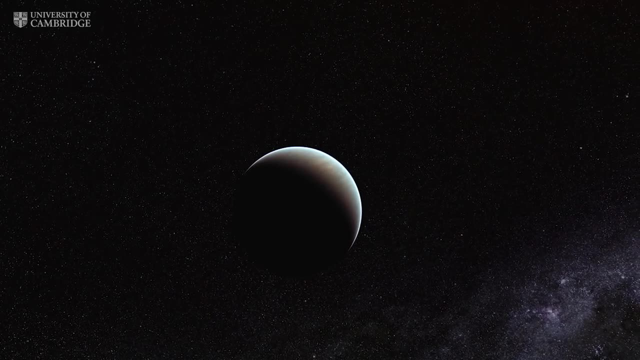 So anything that would tell you there is something going on would be interesting, And maybe one day we'll send a very tiny probe- 100 grams probes- there to take some picture. come back And according to the progress that we have experienced in the last 20 years, 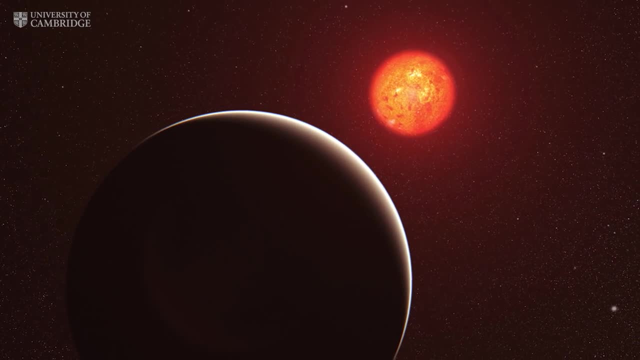 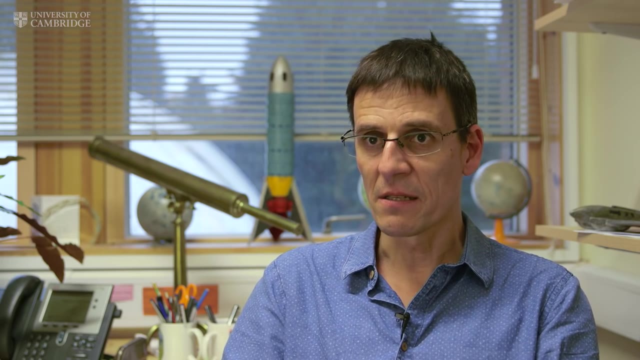 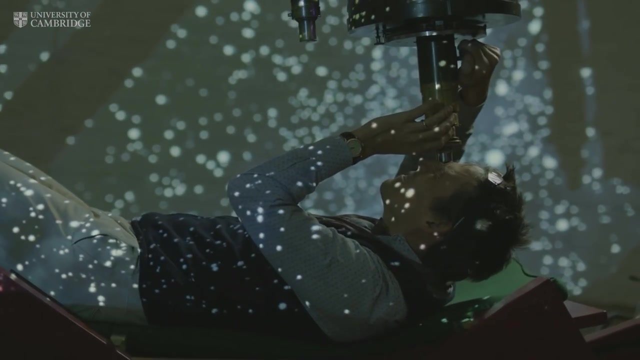 I think there is a lot to hope in the next 20 years coming. Clearly the detections of other planets like the Earth and possibly some hint that there is some interesting species in the atmosphere of some of these planets. I must admit, any time I find a planet on other stars. 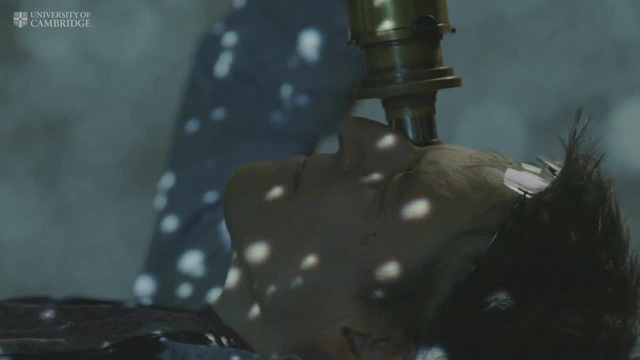 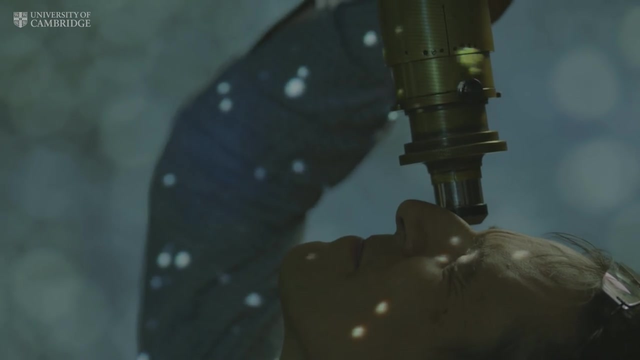 even if right now I should have found more than 200 planets. I feel like a child Because it's like every time, it's a surprise, It's a new system And I keep being surprised, And I used to joke with people asking me about sci-fi movie. 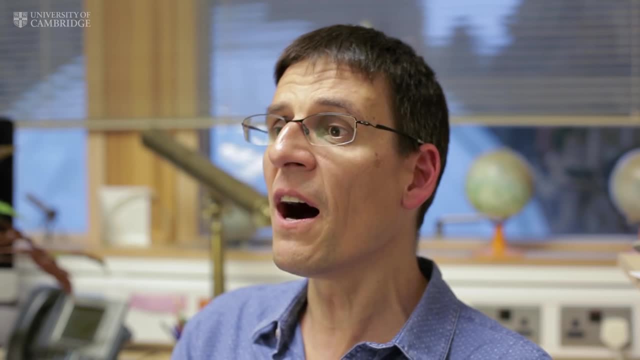 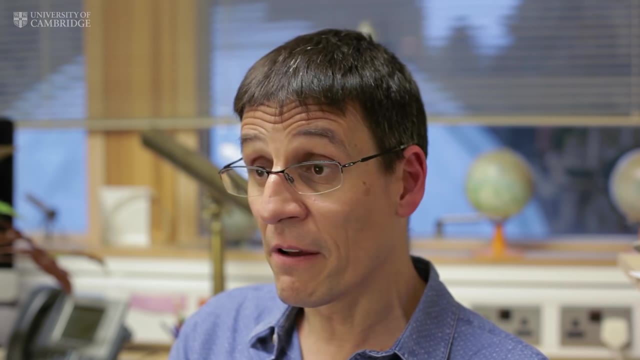 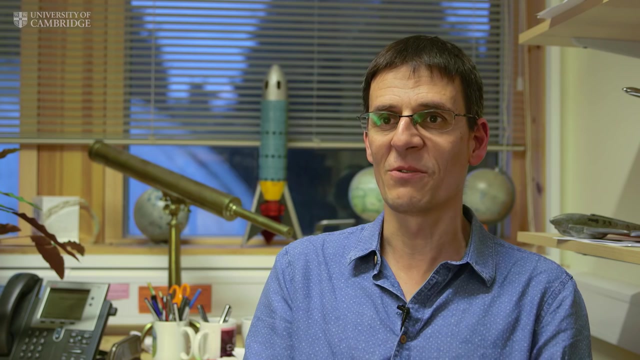 I told them. I mean, the reality is far more exciting and diverse than any sci-fi movie you can have imagined, And I feel very fortunate being surprised like that, And I think this is the purpose of science. So now I think I understand what I did 20 years ago. 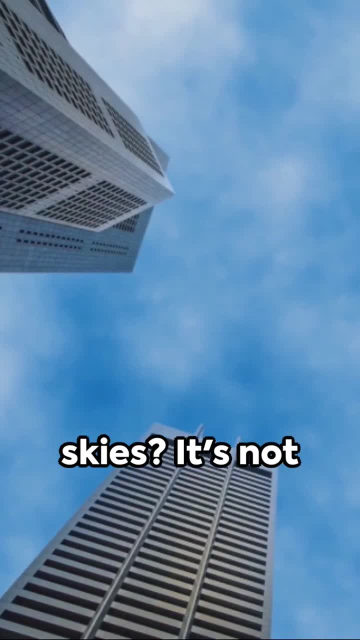 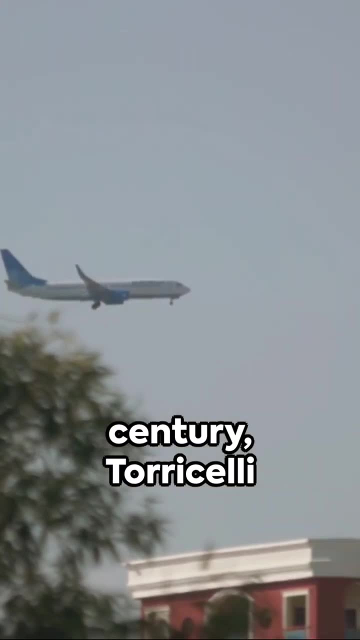 Ever wonder how planes defy gravity and soar through the skies? It's not magic, it's science. Air, a bustling city of molecules, carries weight and creates pressure. In the 17th century, Torricelli discovered this weighty truth. 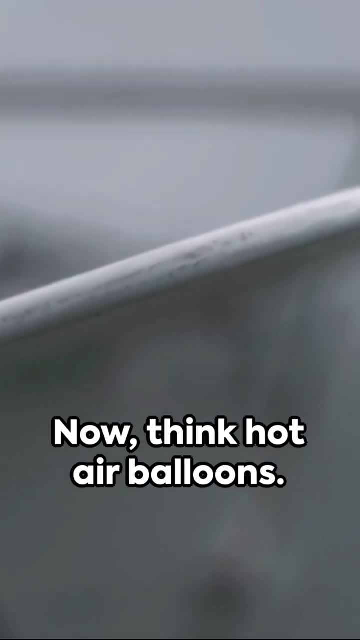 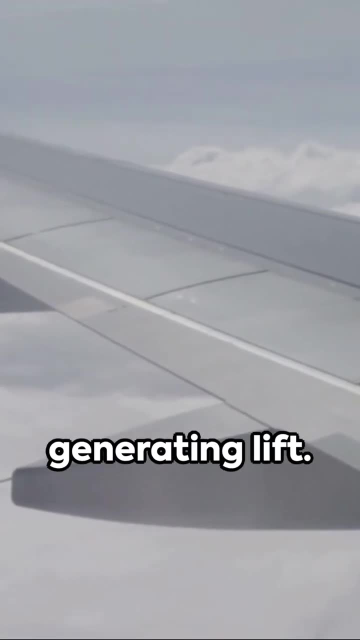 sparking the concept of Lana's airship. Now think hot air balloons. They rise because hot air expands. Similarly, airplane wings are cleverly designed to create pressure differences, generating lift. Four forces play tug-of-war in flight: Lift and wait, thrust and drag. 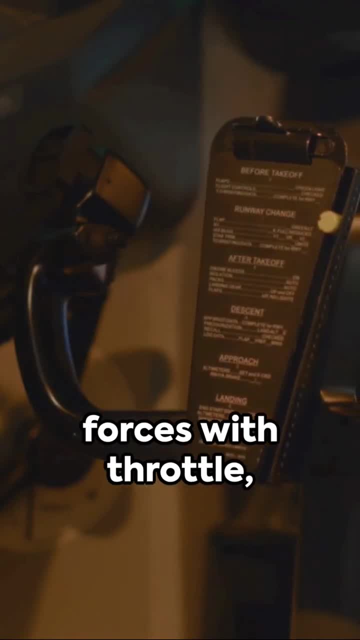 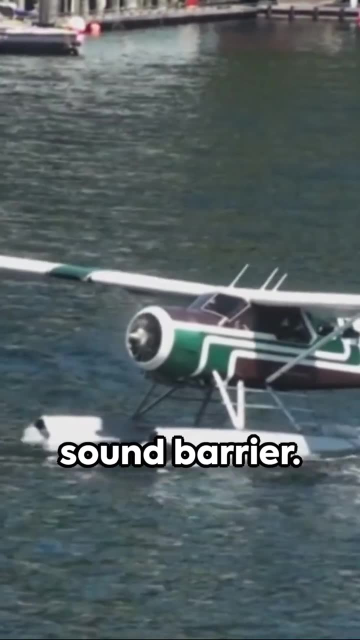 Pilots are the puppeteers controlling these forces with throttle, ailerons, rudder and elevators. From seaplanes to hypersonic rockets, flight speeds vary, crossing even the sound barrier. So next time you're in a plane, remember it's not just a journey.